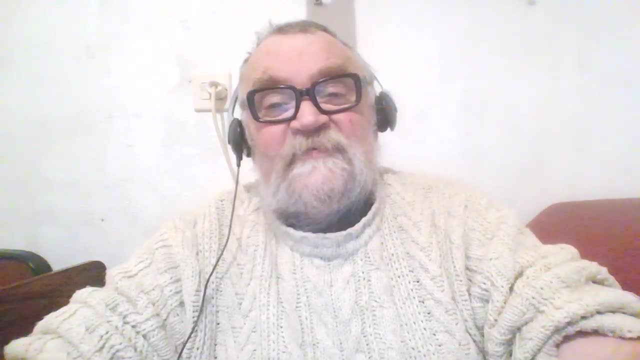 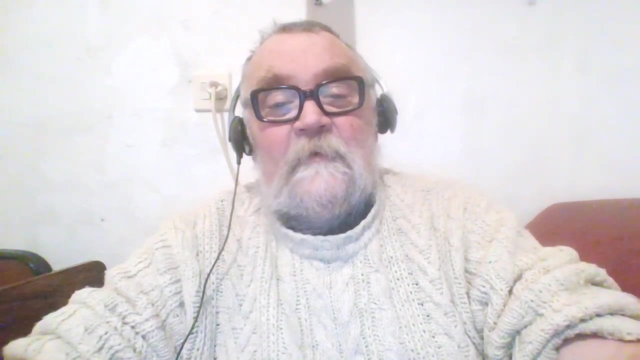 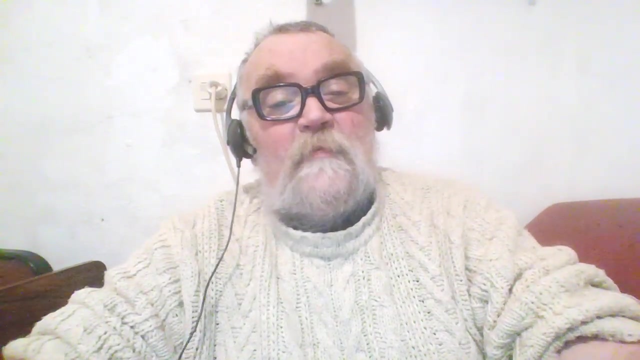 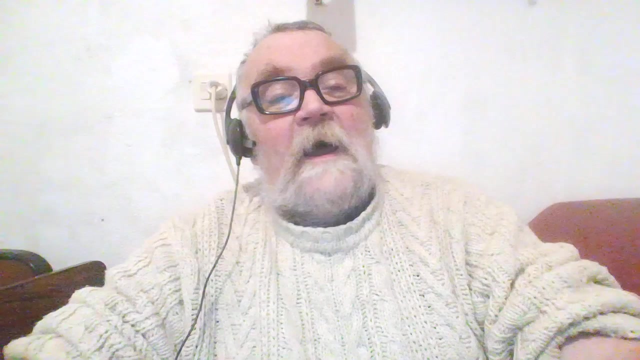 to score. So it's a period of success, a period of good fortune. It's where things are going well, Things are working out. So he was enjoying a purple patch and had scored 12 goals in seven games. I continued my purple patch with a fourth of. 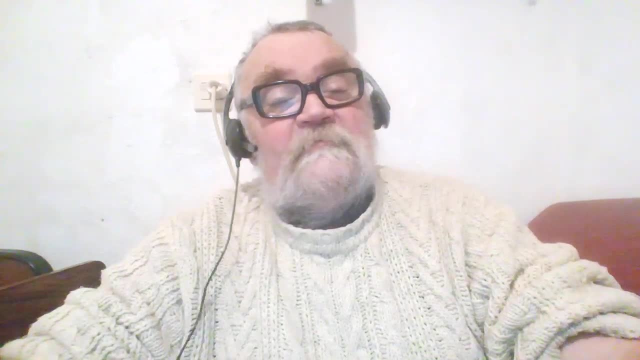 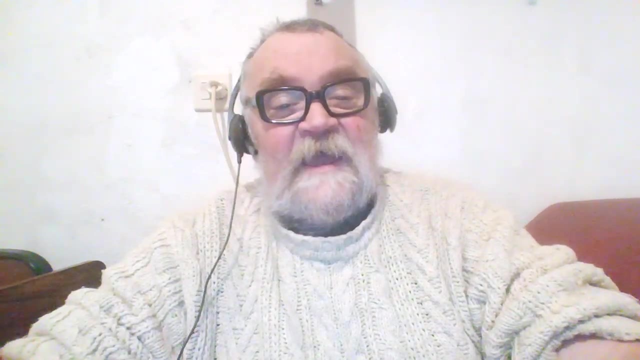 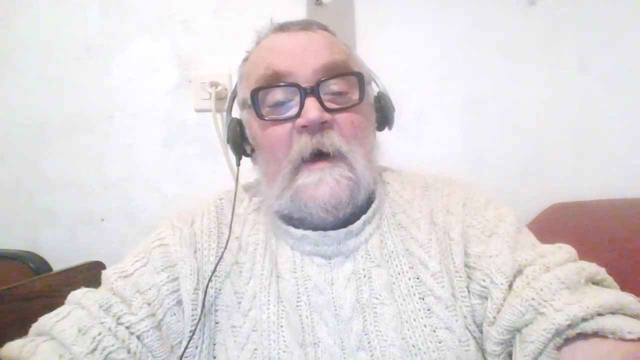 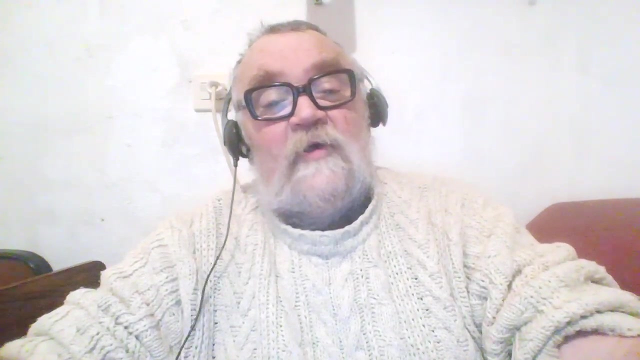 victory. this weekend, My team has hit a purple patch with five victories out of the last six games, So it's a run of success, a run of good luck that things are going well. Yeah, the business is going through a purple patch at the moment. It's gaining lots and lots of clients and it's making loads of money, And this is a 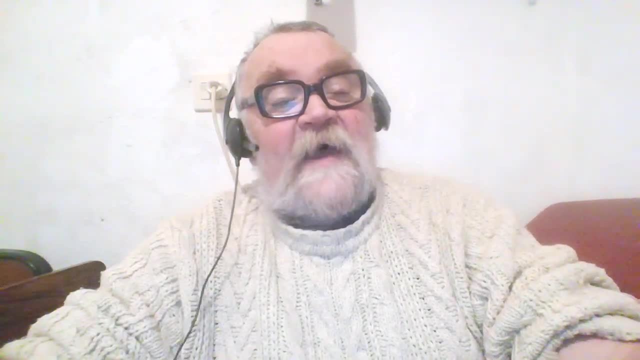 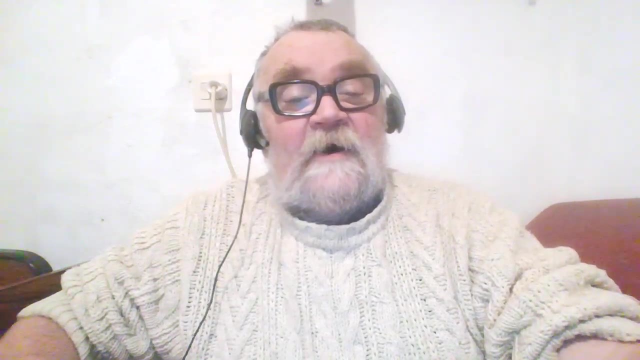 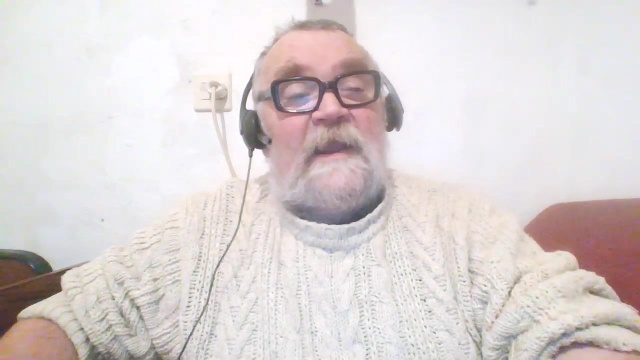 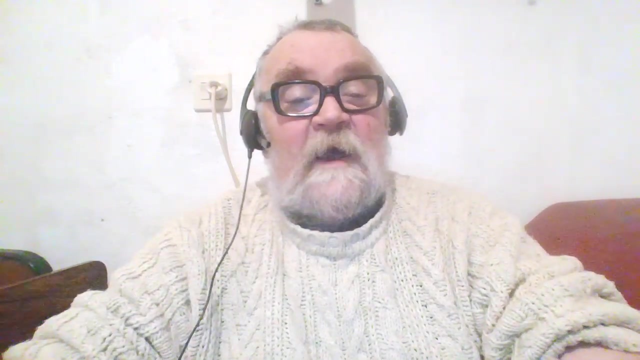 purple patch. If you have a, if you have talented management leading a company, then they are liable to go through a purple patch. Everything seemed to be going well in his life. He found a job, He got a new girlfriend. Yeah, he seems, his life seems to be going through a purple patch. So he's very big, He's. 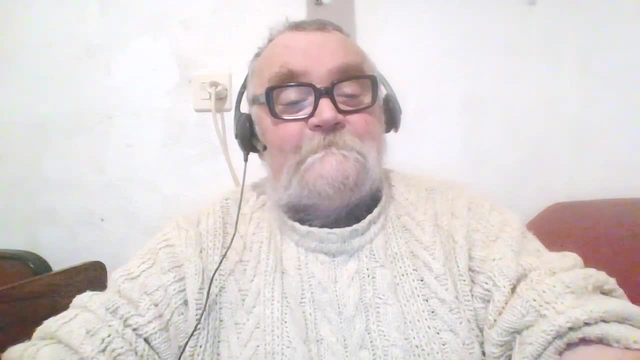 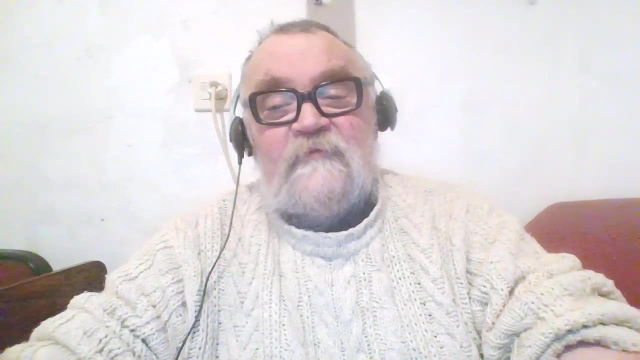 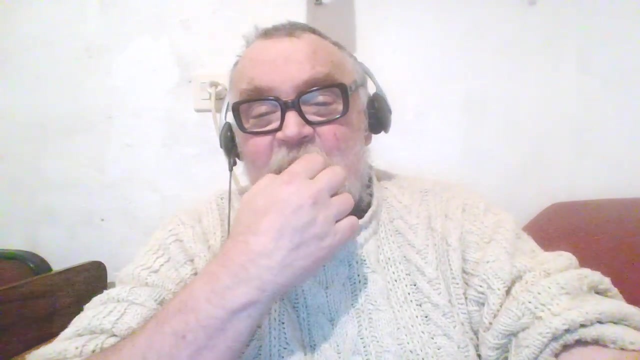 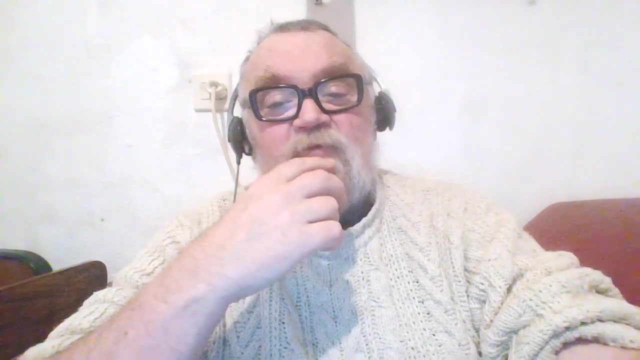 very successful, very successful. Okay so a purple patch, Things are going right, A period of good fortune, Everything's going in the right way. Let's see This comes from purple pros. Let's see, Purple pros- I've got a video about this- is writing, which is extremely elaborate, incredibly elaborate. 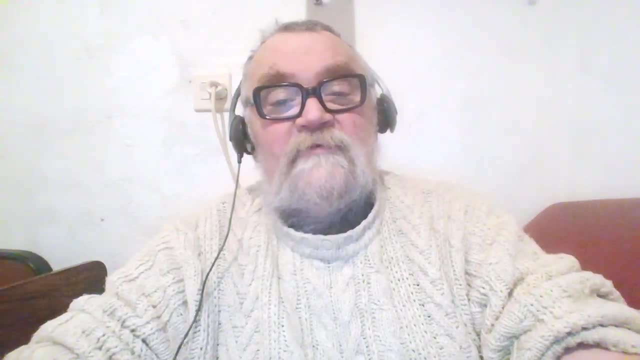 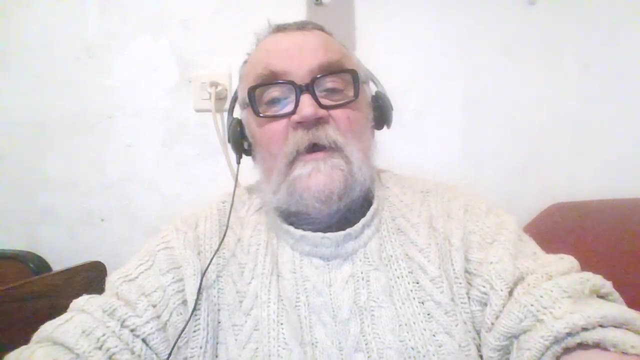 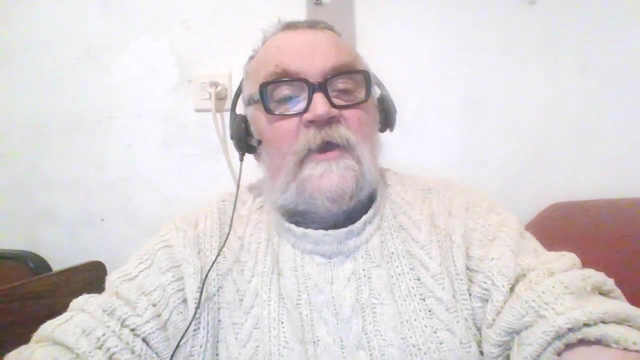 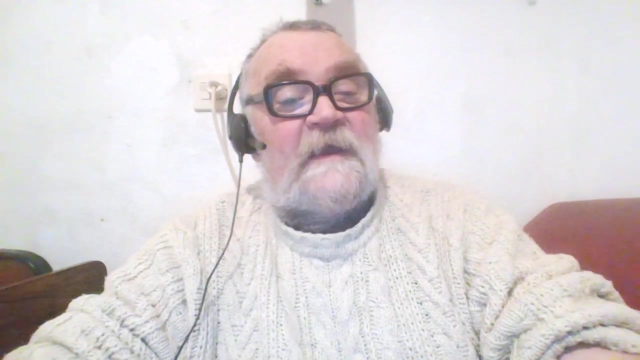 descriptions, And this purple pros actually comes from the Roman poet Horace Kintus, Horatius Flaccus, And in one of his works he says: your opening shows great promise and yet flashy purple patches, as when describing a sacred grove or the altar of Diana, So purple.